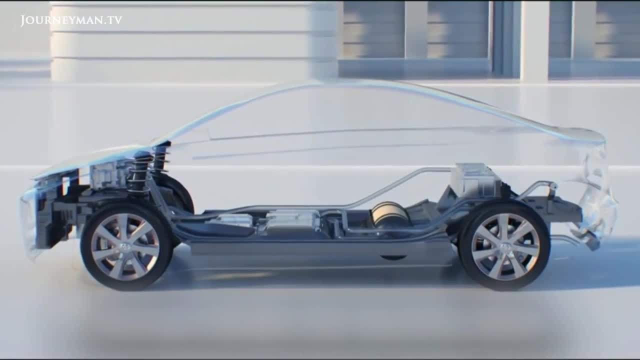 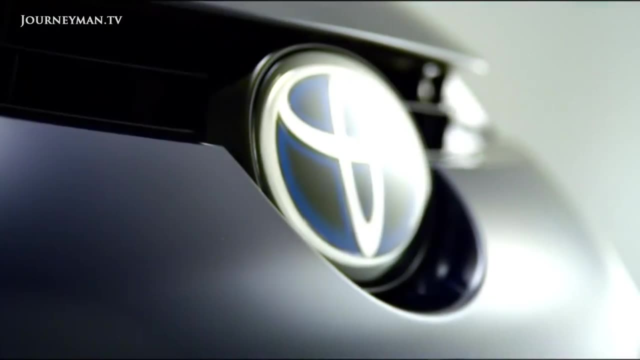 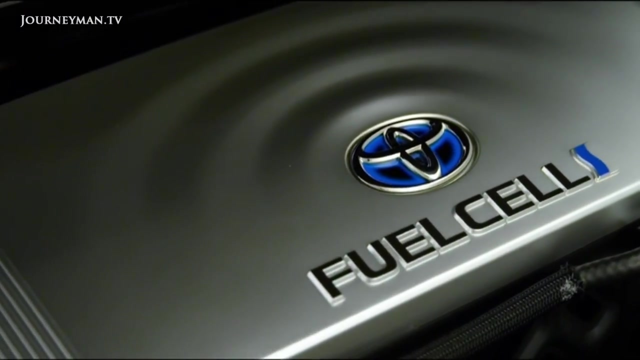 And two giants of the motor industry have already adopted the technology. The revolutionary Toyota Mirai is the world's first mass-produced fuel cell saloon vehicle powered by the Toyota fuel cell system. Japanese automotive manufacturer Toyota tested its hydrogen-powered Mirai in the United Arab Emirates. 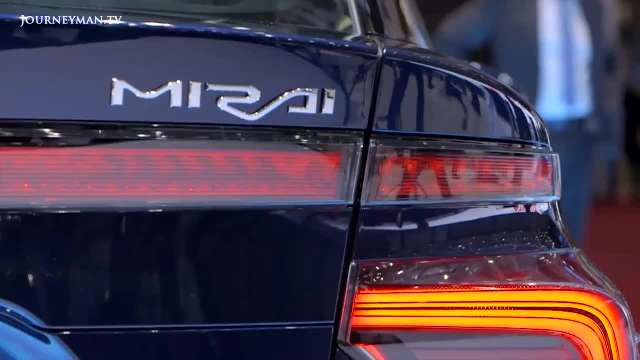 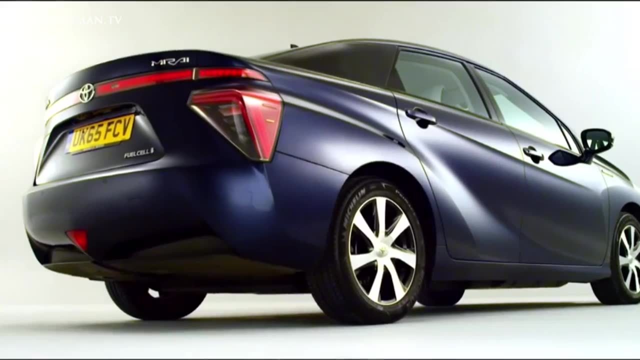 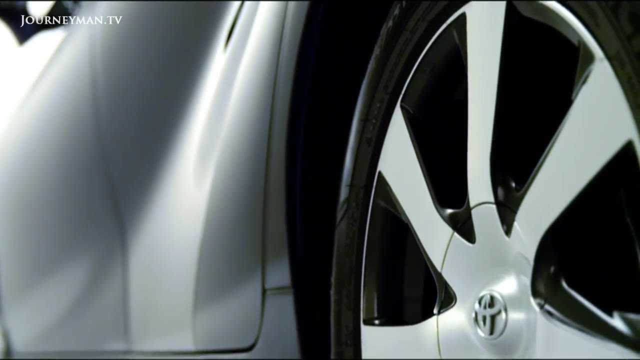 The region's hot and arid landscape allowed the company to measure the effectiveness of the hydrogen-powered Mirai. However, it's not a solo venture. The company will be partnering with UAE-based green energy companies as well as utility providers, to get a realistic grasp of the logistics of implementation. 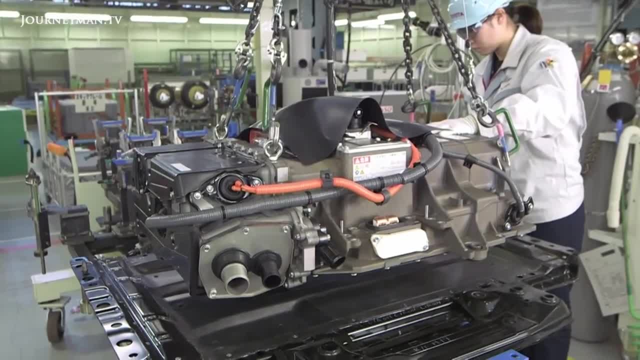 And they're not the only company worried about reducing their carbon footprint. Hyundai is committed to improving the environmental impact of our vehicles. The company is committed to improving the environmental impact of our vehicles. The company is committed to improving the environmental impact of our vehicles. 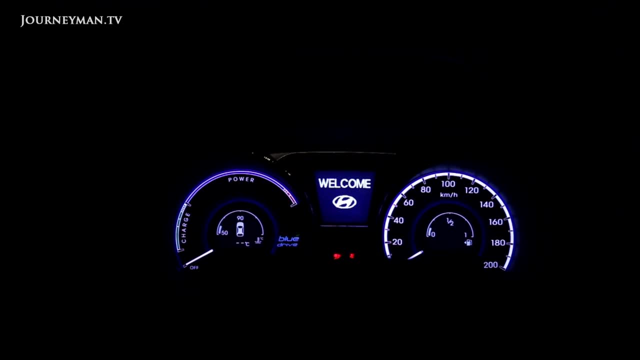 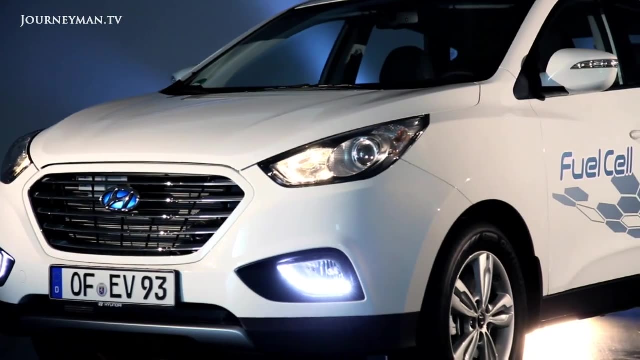 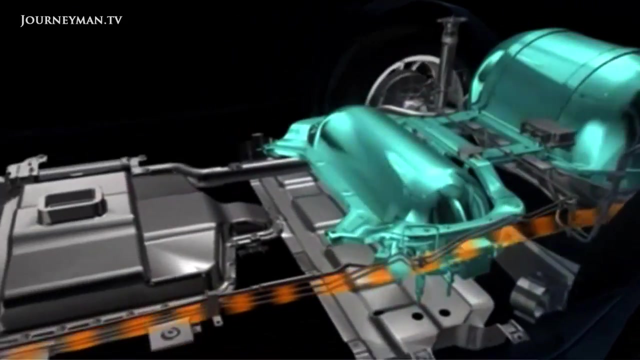 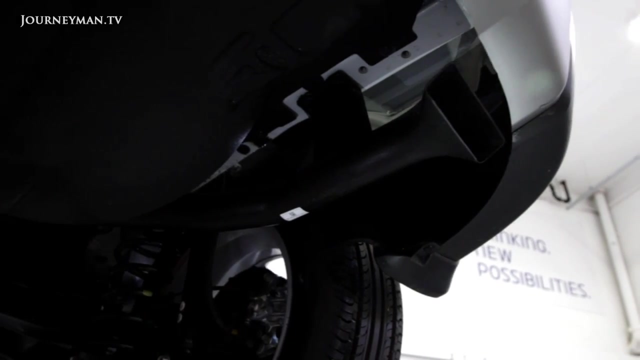 The car from Hyundai was the world's first production model hydrogen fuel cell vehicle. The company boasts world-leading zero emissions technology and they believe the innovation takes a giant but viable step towards an alternative to the internal combustion engine, And Hyundai have even promised the smoothest ride ever. 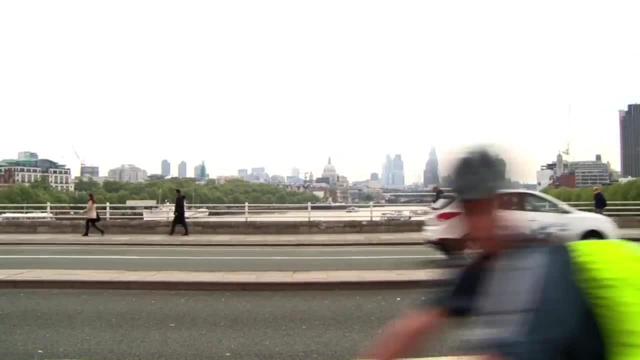 The world's leading initial production aircraft for the hydrogen naturally-fueled fuel cell was Hyundai's��는 Hyundai X35 fuel cell. The story tho? o has been already played out in the short film that was developed by Hyundai, and Hyundai Sees itivil explains technology. 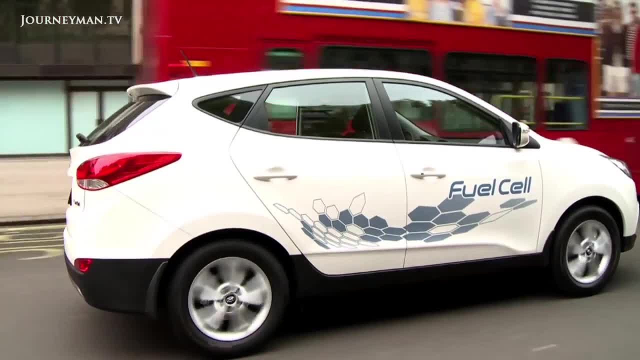 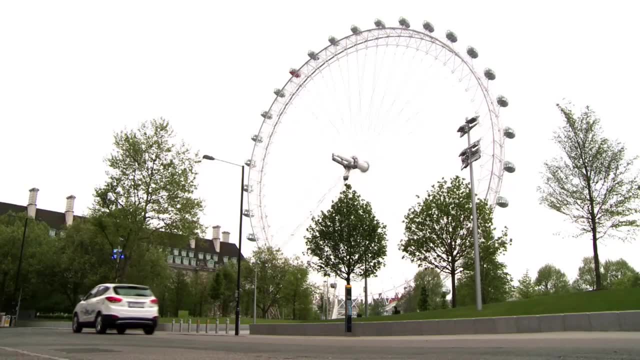 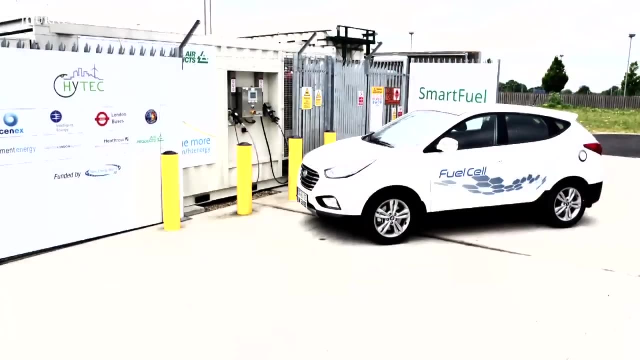 comparable with conventional diesel or petrol technology, are far in advance of current EV technology, And the 100-kilowatt fuel cell stack and 24-kilowatt battery can also reach a top speed of 100 miles an hour. However, it isn't just on the roads. 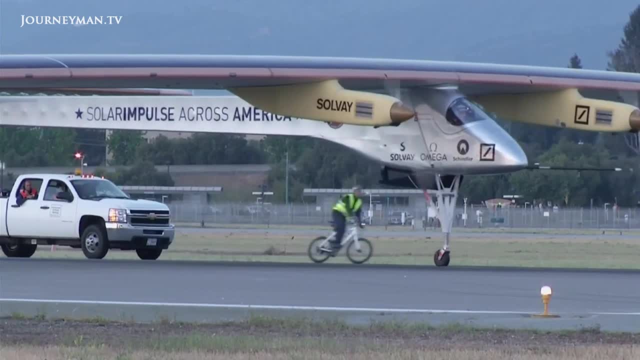 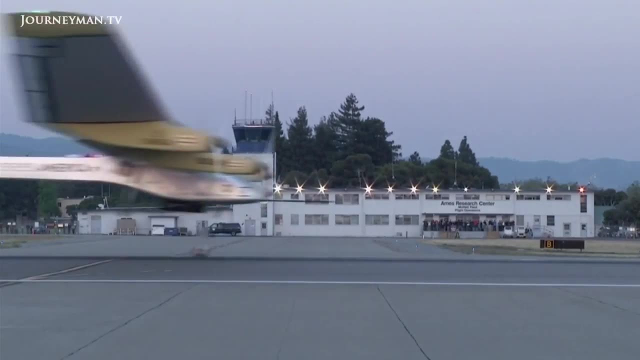 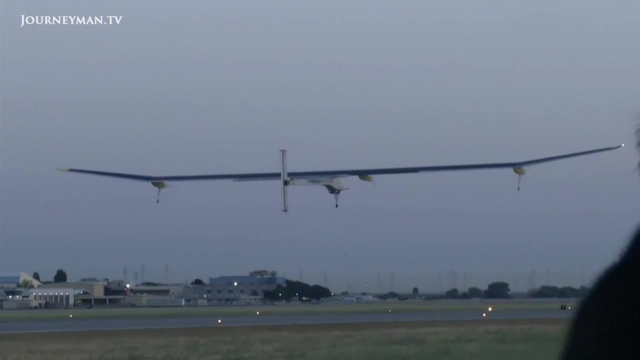 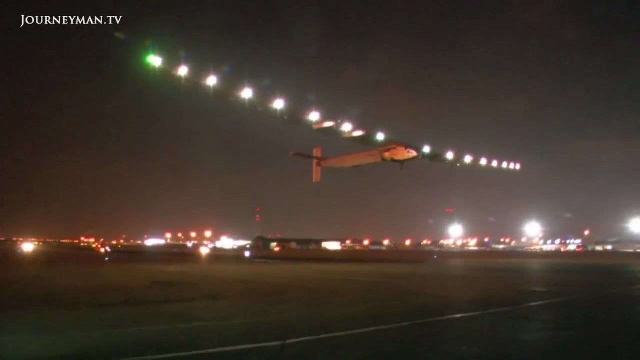 where the future of green travel has been implemented. There have also been some significant developments in aviation. Last year, the Solar Impulse completed an impressive round-the-world trip using solar energy. The plane traveled over 40,000 kilometers, visiting the UAE, China, India, Japan, USA, Spain and Egypt. 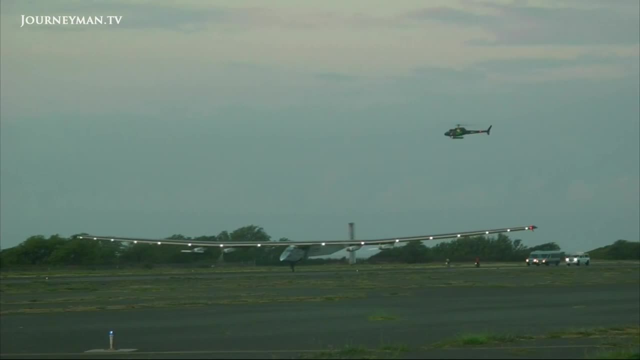 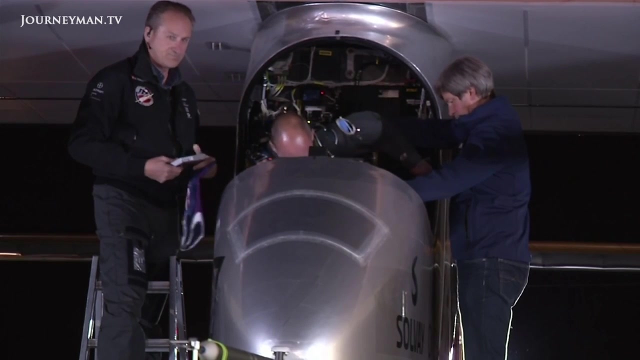 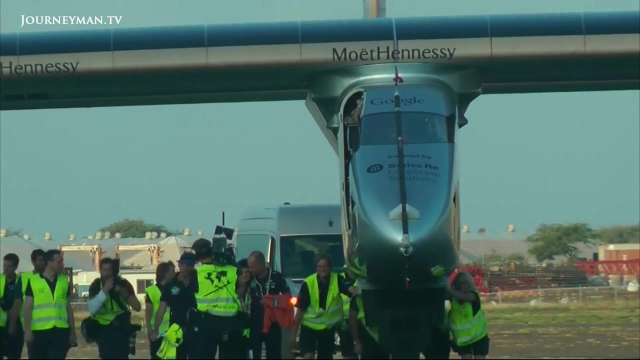 all without using a single drop of fossil fuel. In March 2017, the European Union announced it will partner with the team that made the first solar power plant, And the collaboration hopes to come up with 1,000 energy-efficient solutions by the end of 2018.. 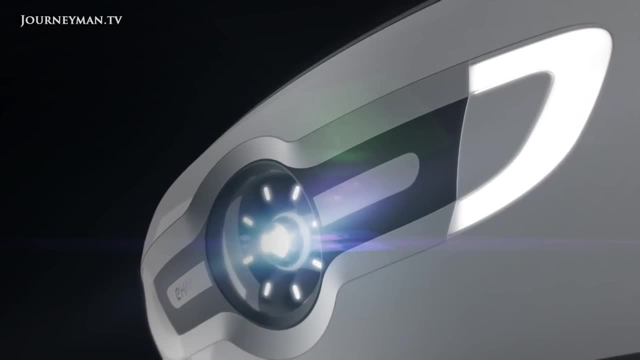 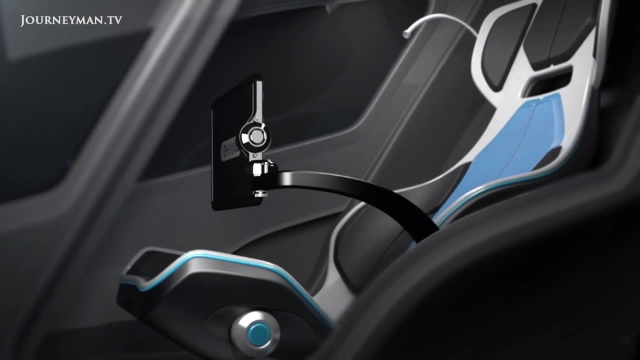 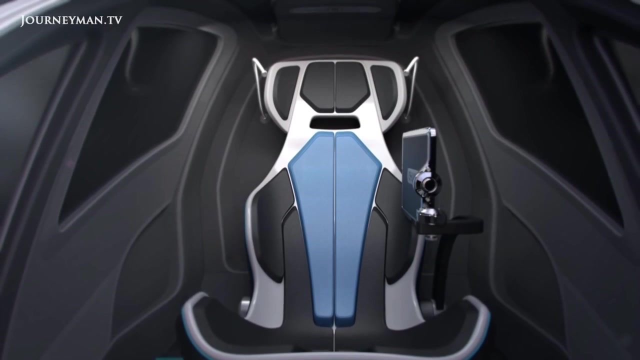 However, surprisingly, it's not just planes that are flying With roads around the world getting busier by the day, some companies are working on innovative solutions to help people beat the traffic. Recently, it was announced that Dubai, which is a major city, 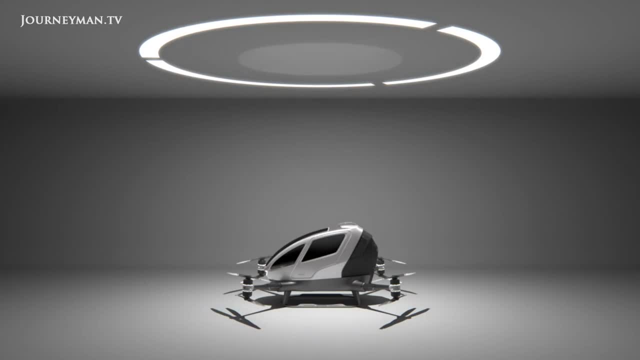 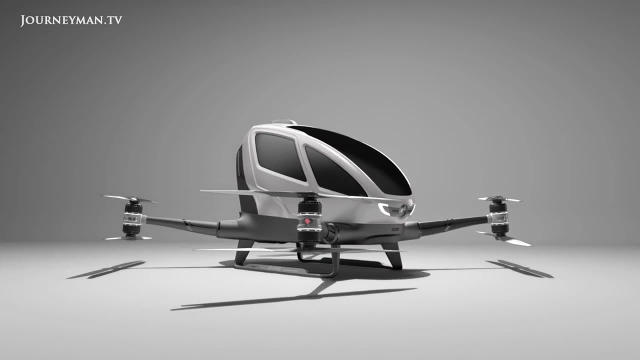 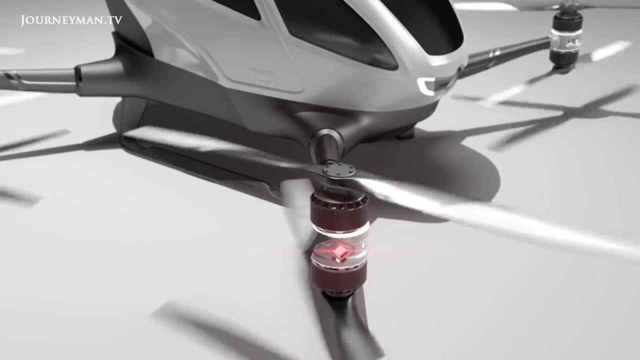 has become a top destination for the mobile industry. Dubai has carried out test runs of a one-person electric flying car. The new e-hang 184 has successfully flown across the city. The company claims passengers don't even need a pilot's license. 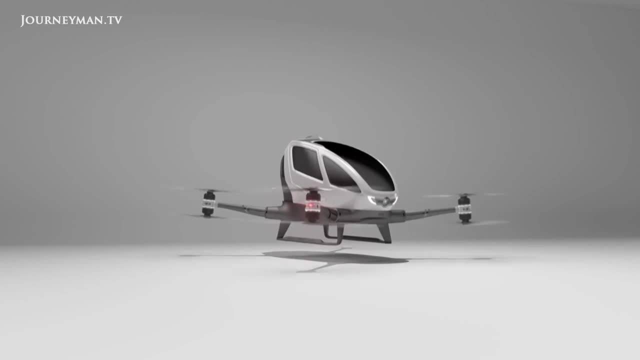 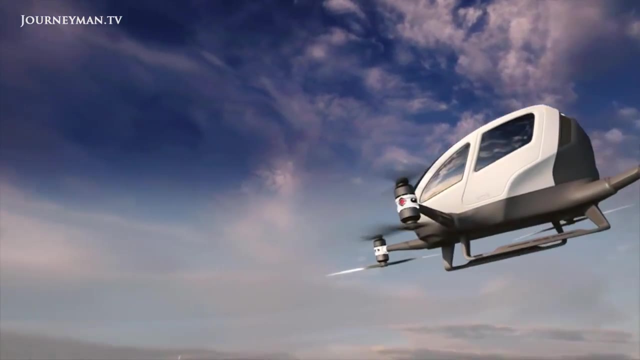 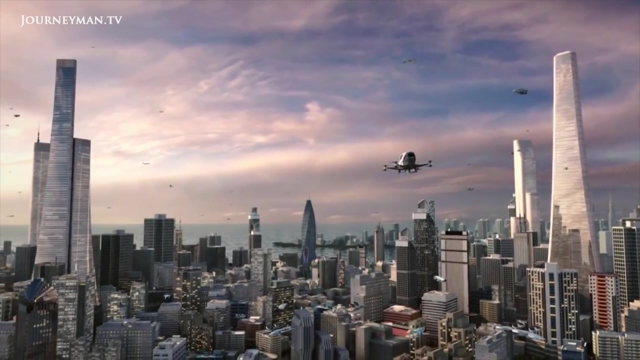 as the automated vehicle is operated. by the press of a button, The vehicle takes off vertically, gliding through the air as it transfers fuel to the engine, which will then be supplied to the fleet, transports passengers from point A to B. But they're not the only company pioneering this new technology. 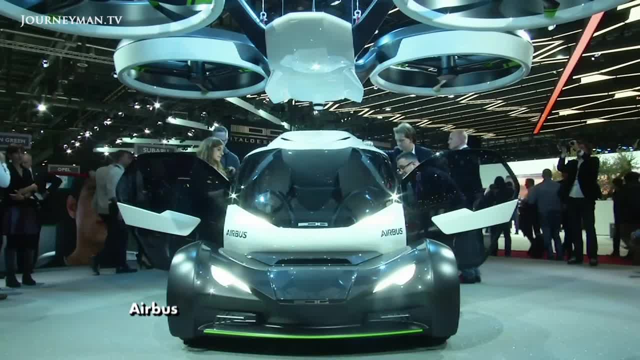 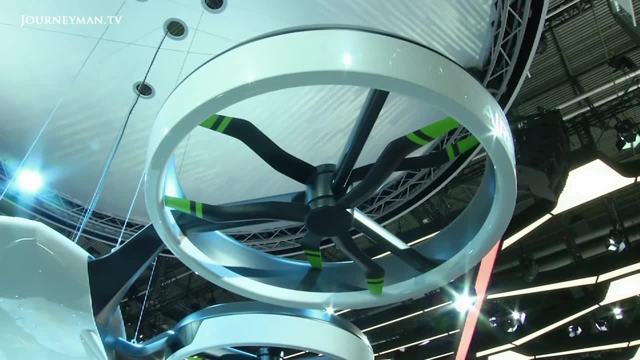 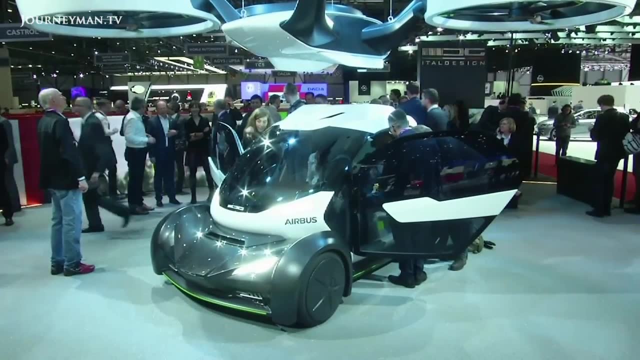 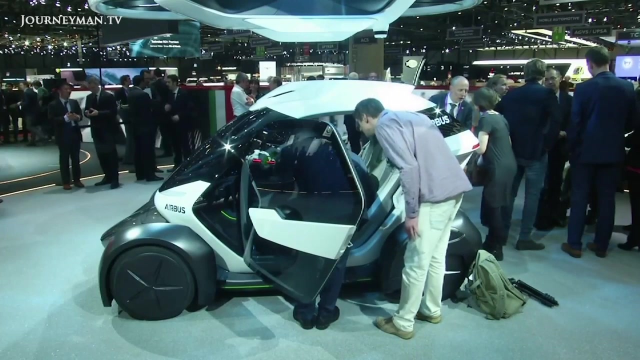 At the 2017 Geneva Motor Show, Airbus unveiled their pop-up flying car concept, And the modular air and ground passenger vehicle consists of three main components: A carbon fibre passenger capsule, battery-powered ground module and an air module electrically propelled by eight counter-rotating rotors. 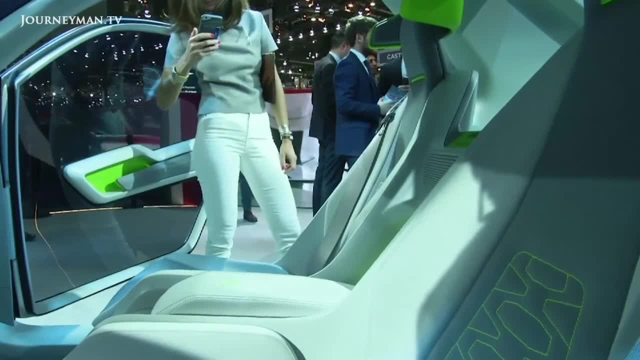 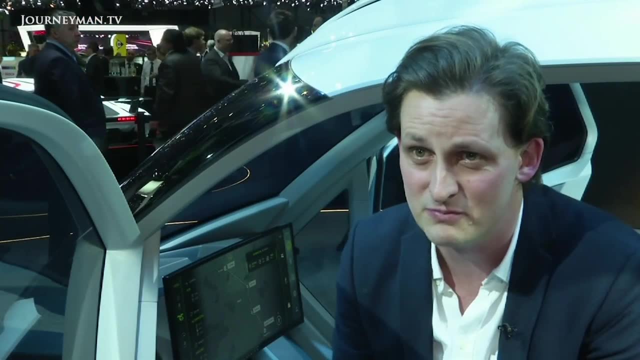 General Manager at Airbus Urban Mobility, Matthias Thomson, is excited about what it means for the future of travel. I think it'll be incredible. You're in your capsule, You don't have to go in and out, It's integrated, it's seamless. 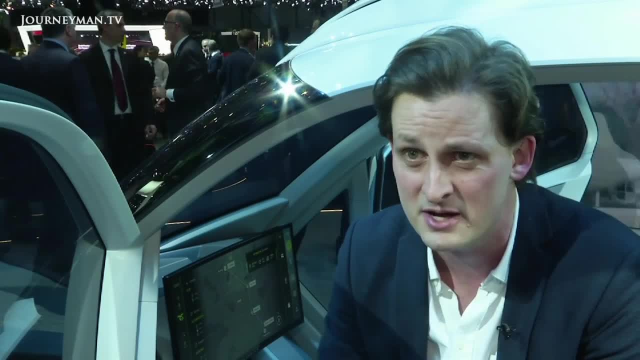 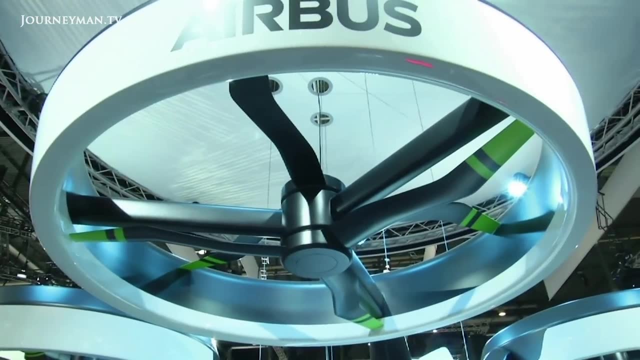 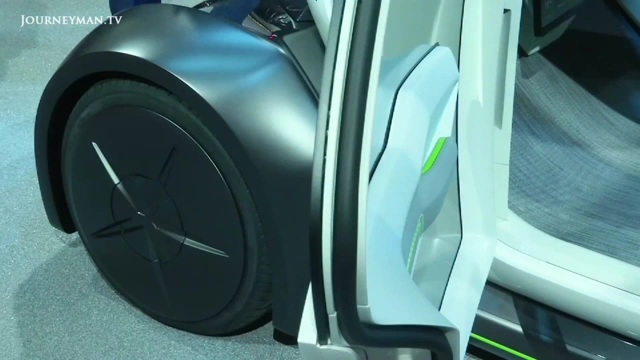 It'll be the most pleasant way of getting around town, getting to the airport. I think it will irresistibly nice. Passengers will be able to plan their journey and book a flight using a simple app. The system then suggests the best mode of transport.